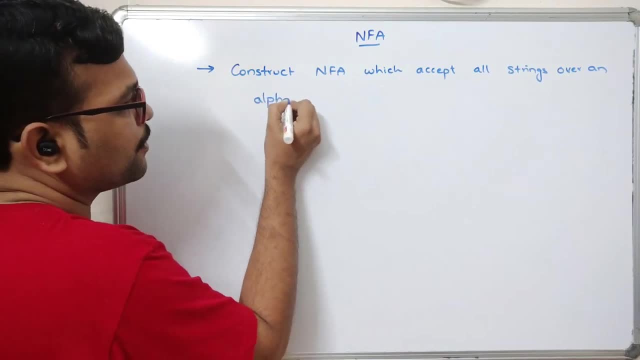 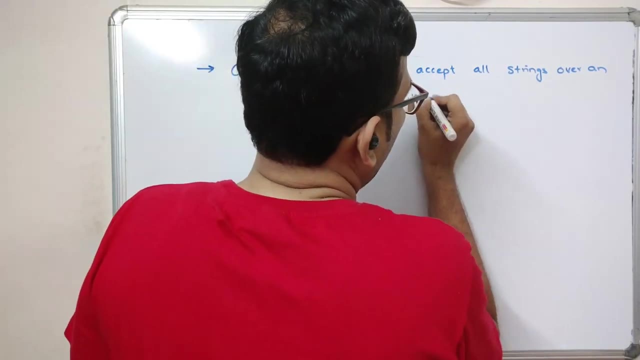 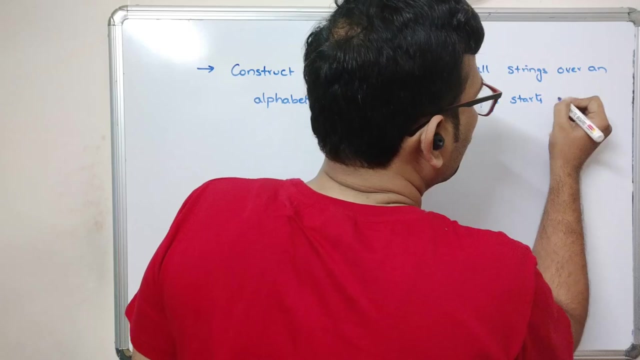 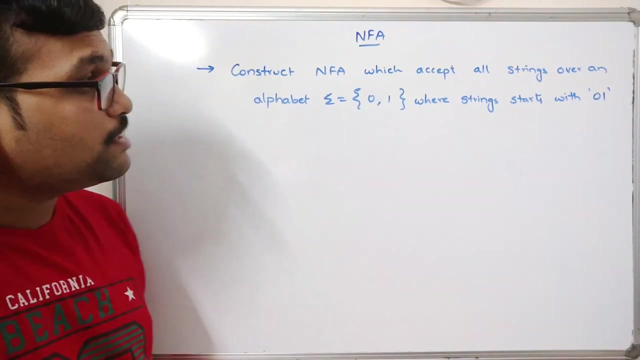 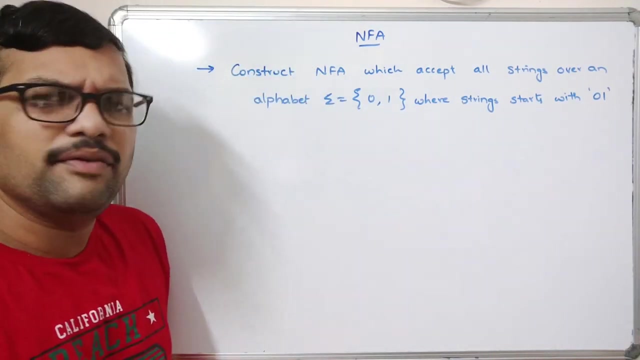 sigma is equal to 0, 0 and 1, where strings starts with 0- 1. here we need to construct the NFA which accepts all the strings over an alphabet. this thing starts with 0- 1 and let it be whether it can be DFA or NFA. first step we need to write the language. So language is equal to 0, 1 and 0, 2.. Let us cell now. There is a set of two formulas here. We need to run one, Ник Но, to make one of themhl. and next step here, say you will: 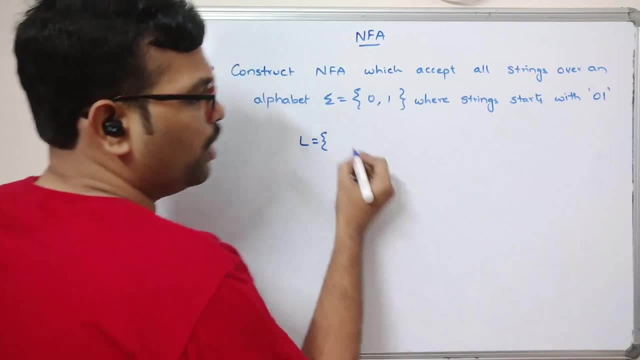 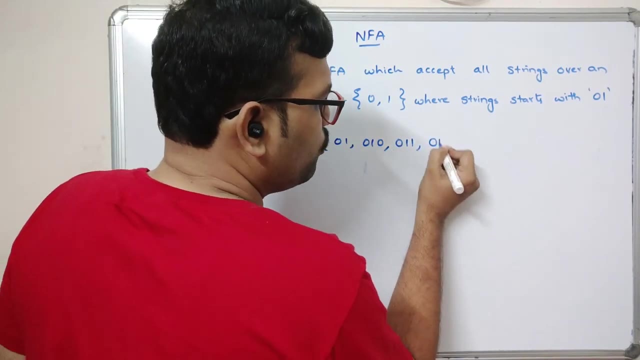 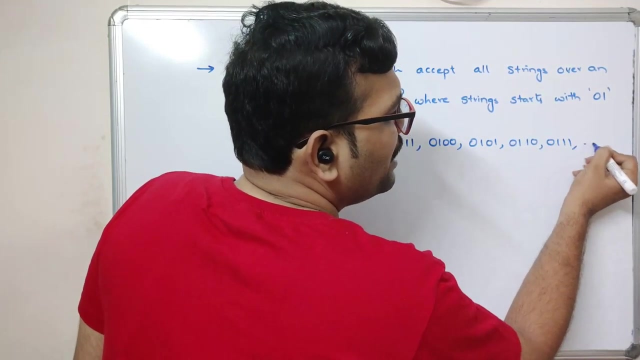 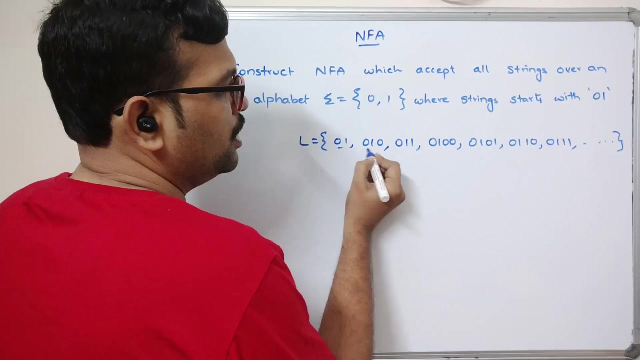 all the accepted strings Depends which strings starts with 0, 1.. So 0, 1, sorry- 0, 1, 0, 0, 1, 1, 0, 1, 0, 0, 0, 1, 0, 1, 0, 1, 1, 0, 0, 1, 1, 1, and so on. So this is also an infinite language. So here you can observe: in all these strings the string starts with 0, 1.. So in all the strings the string starts with 0, 1,. right Now let us consider the same. 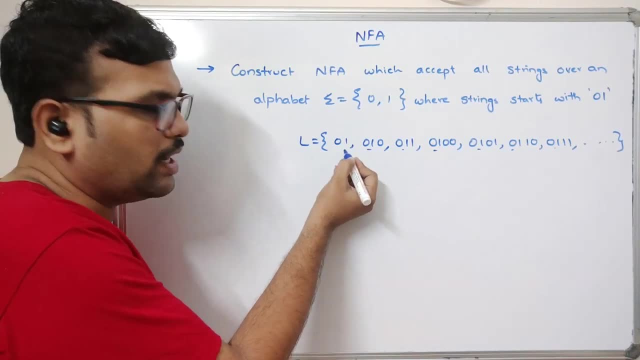 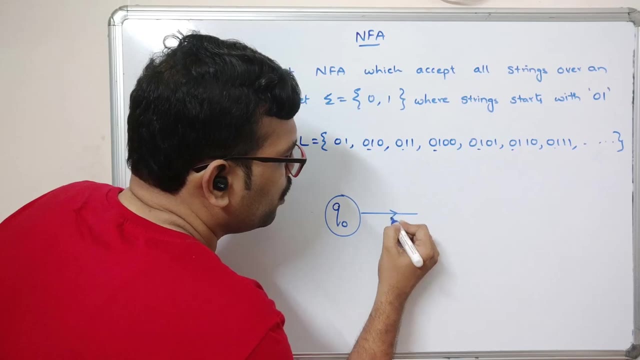 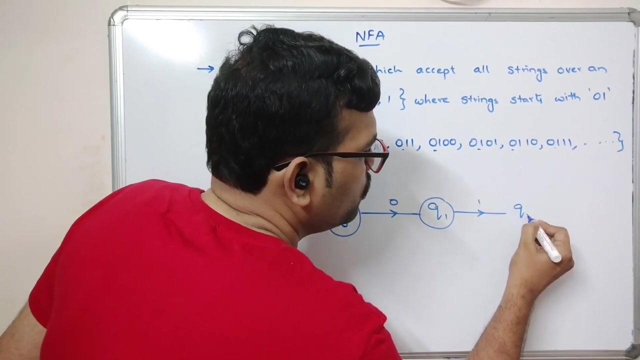 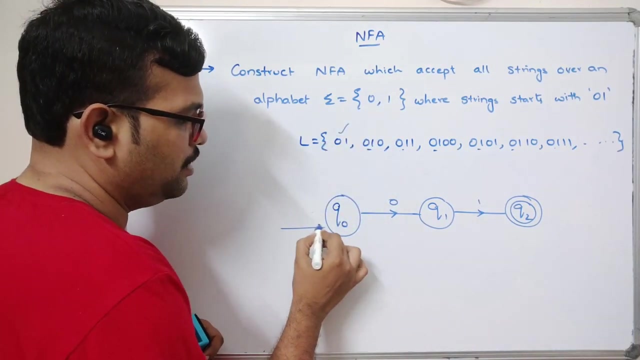 procedure. So first we take the first string, which is of the length 2.. So we require three states here. So simply go with a q naught, and q naught upon 0 move to q 1, q 1 upon 1 move to q 2, and you can observe here: So this one is a satisfied and this is an initial. 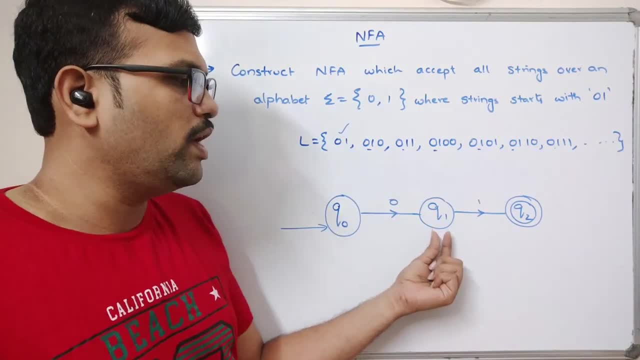 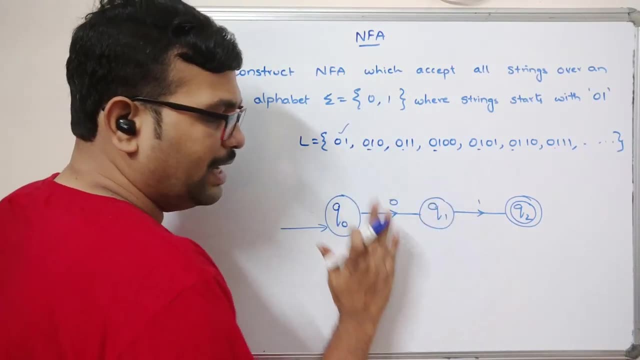 state. This is an initial state, and upon 0 it moves to q 1, and upon 1 it moves to q 2 and q 2, and here see 0, 1, this one satisfied, and what about this one? 0, 1, 0.. So always. 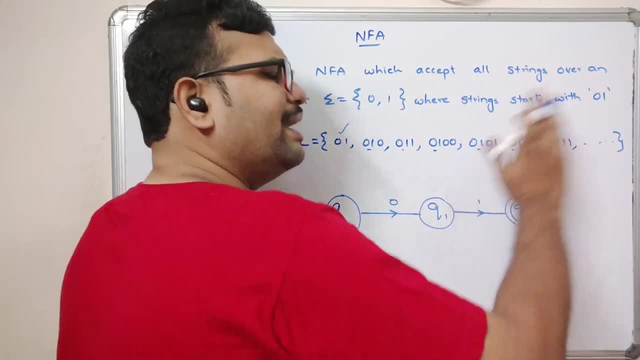 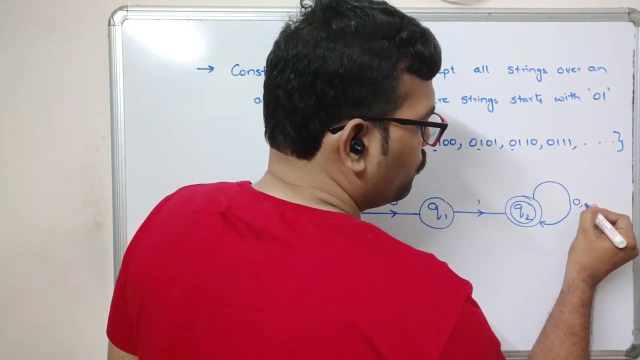 it should start with 0, 1 and after this, 0, 1, n number of 0s and n number of 1s can be appeared. So simply you can give the self transition for 0 and 1, right, 0 and 1. and. 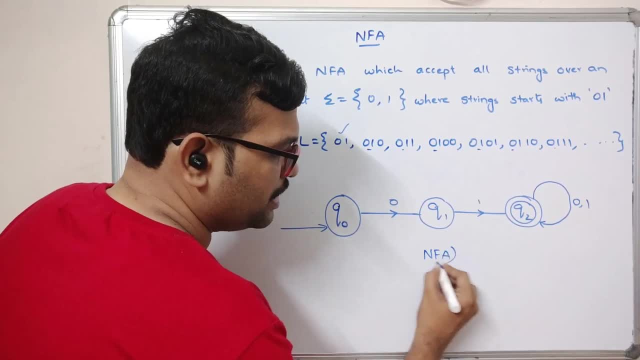 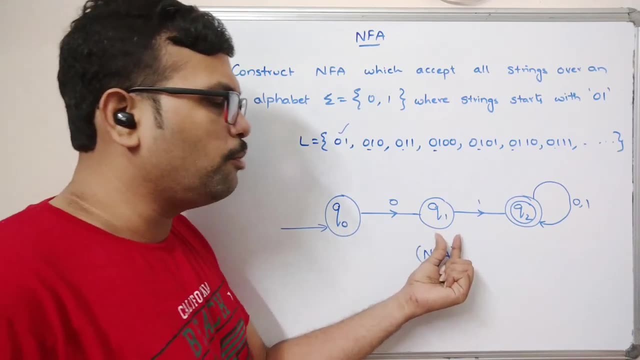 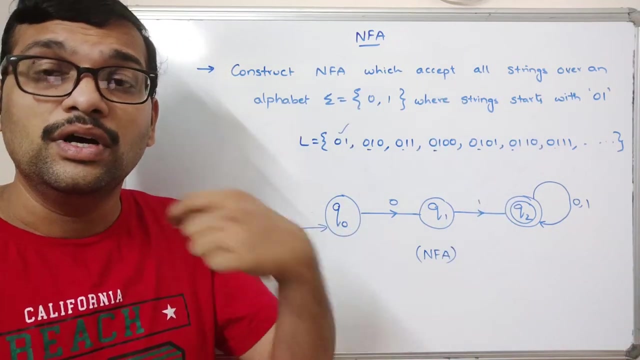 this is the NFA. This is the NFA, So you need not bother about the transition over q naught on 1.. Here you need not bother about the transition for q 1 on 0. So there is no restriction that every state should have the transition. So the state can have the transition or may not. 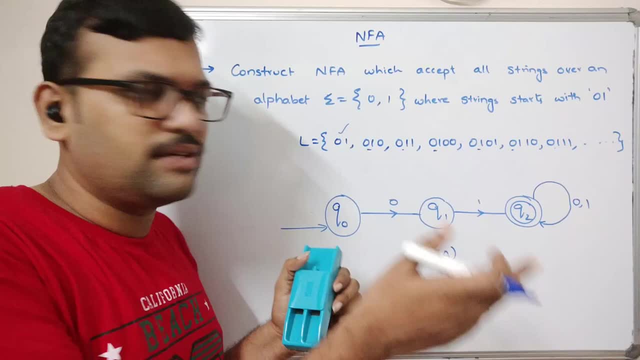 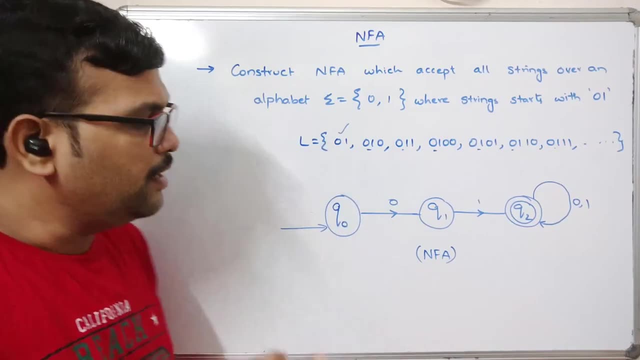 have the transition right. If it is required, we can have the transition from one state to another. If it is not required, we need not use the transition over the alphabet, right. So here you can see: if the string is 0, 1, so q naught on 0, it moves to q 1 and. 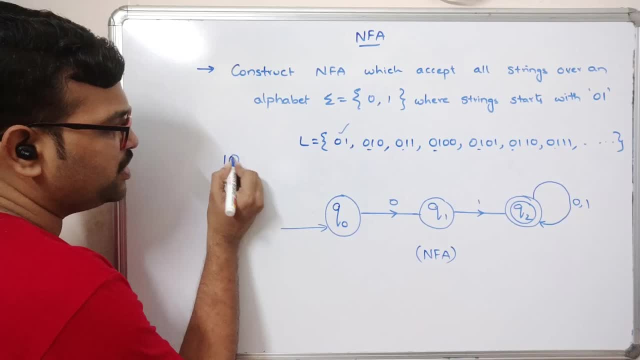 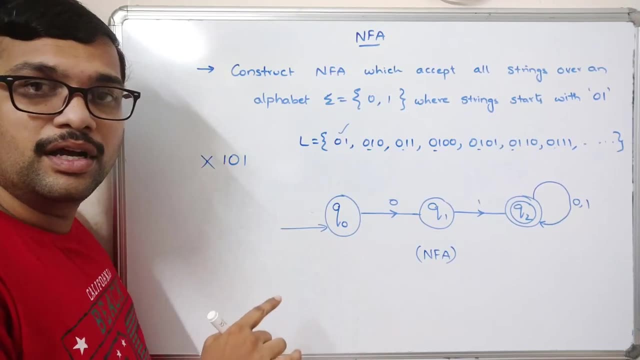 q 1 on 1, it moves to q 2, that is it. If it is 1 0 1, you can observe q naught on 1, there is no transition. So this string itself will be rejected by this NFA. So we need not bother about the q naught on transition. 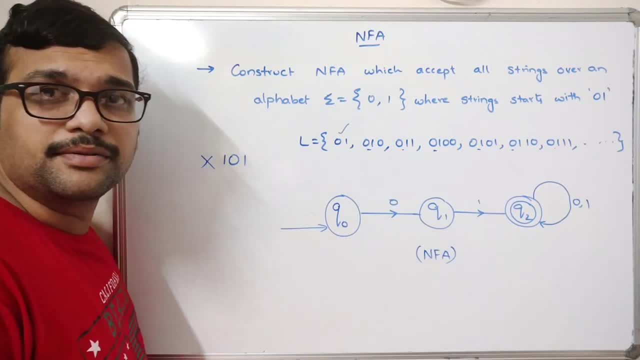 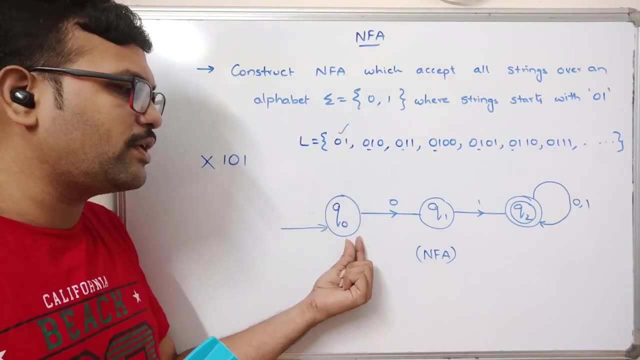 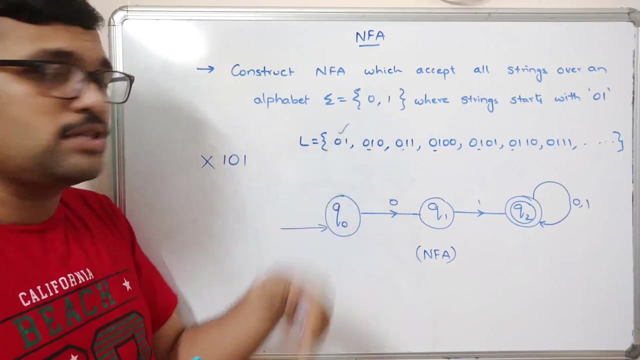 1 because it is not a valid. So simply you can eliminate, right. So this is called the NFA, So in DFA. so we have to give the transition for q, naught over 1, right For every state. there should be a transition for the input symbols, one transition for the input symbols. 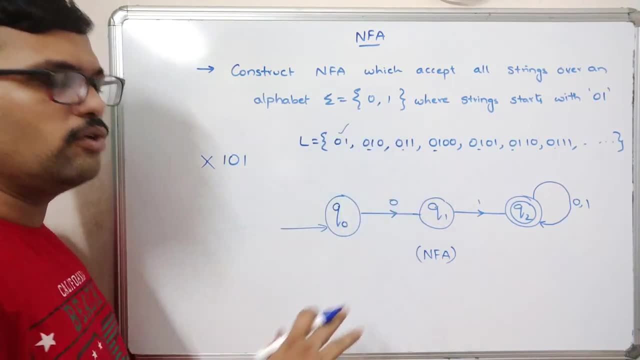 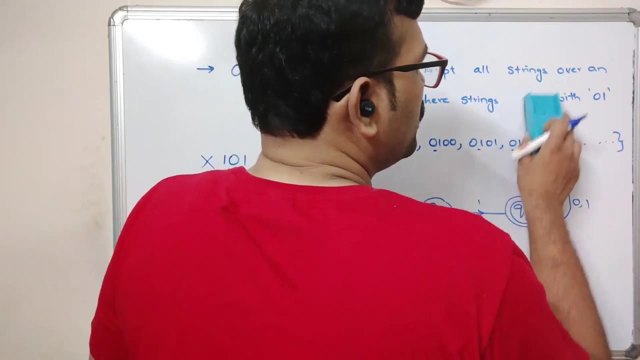 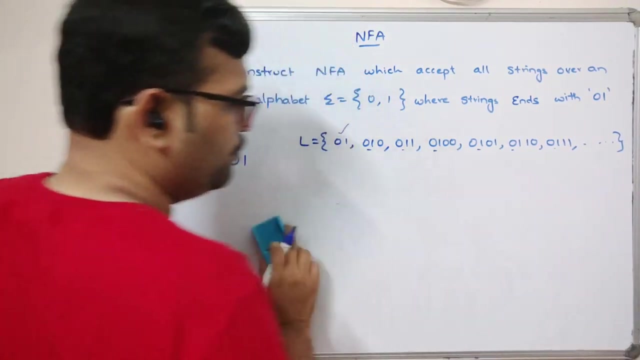 right, That is a DFA. And coming to the NFA, you need not give the transition for every input symbol, right? So this is a small example and one more example. if you go with the ends with, If you see the example ends with, ends with 1, 0, 1, ends with 0, 1.. So let us let me write the language. 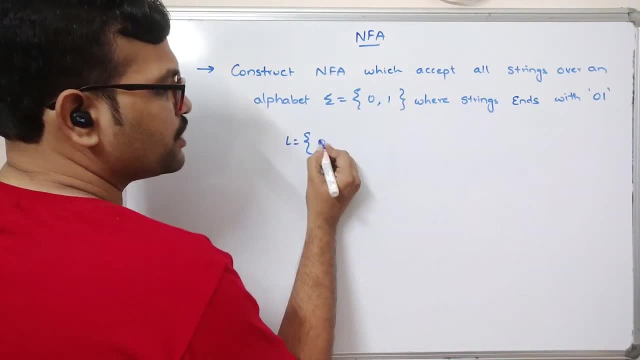 first. So L is equal to ends with 0: 1,. the first one will be 0: 1, and here the strings should ends with 0, 1 and the strings can start. So L is equal to ends with 0: 1,. the first one will be 0, 1, and here the strings should ends with 0, 1 and the strings can start. So L is equal to ends with 0, 1,. the first one will be 0, 1, the strings can start. So L is equal to ends with 0, 1, the first one will be 0, 1 and the strings can start. 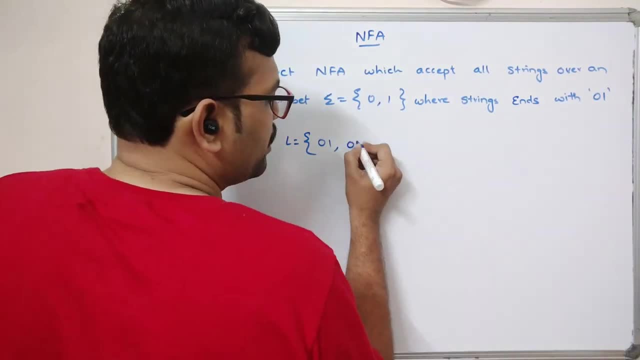 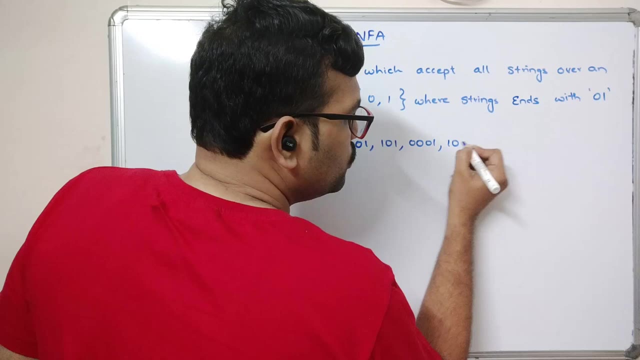 with any number of ones and zeros, right, So let me write the here. So 0 0 1 and 1 0 1 and 0 0 0 1 and 1 0 0 1, 0 1 0 1, 1 1 0 1 and etc. 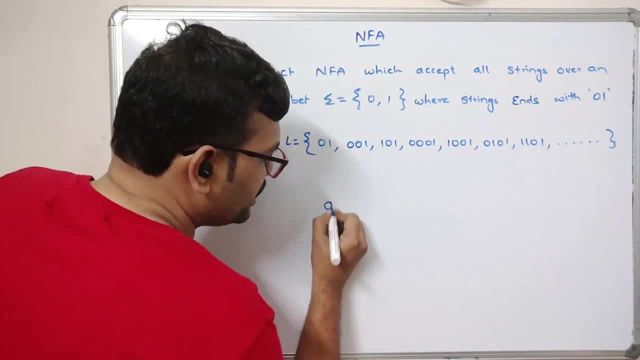 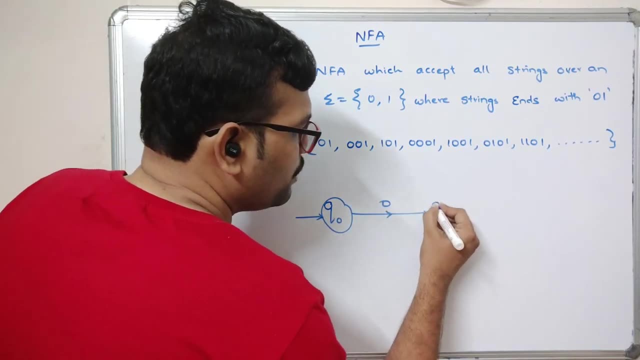 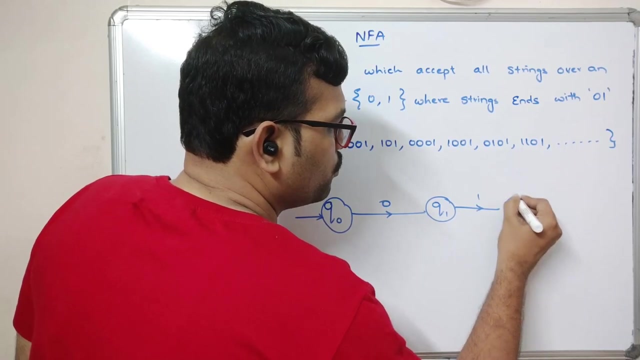 So this is also an infinite language. right Now, let us take the state q naught, which is the initial state. So q naught upon 0, it moves to q1 and q1 upon 0.. on 1 it moves to q2, which is a final state. now, here the question is: ends with 0- 1. so